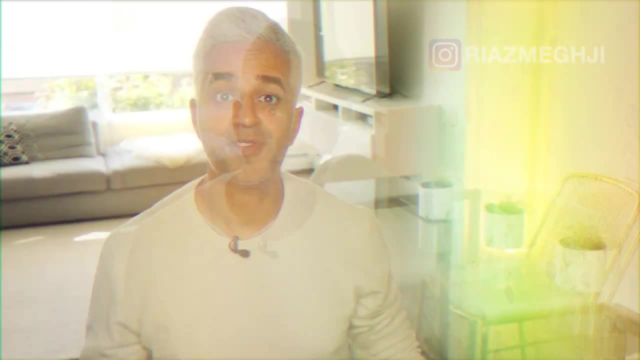 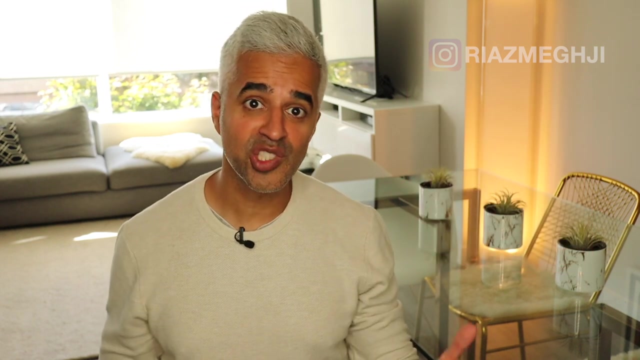 help you successfully speak impromptu. First off, ask who. Who are you speaking to? Is it a formal audience that wants a serious tone, a casual audience that just wants to laugh and have fun, fun, or a group of leaders that wants to be inspired? 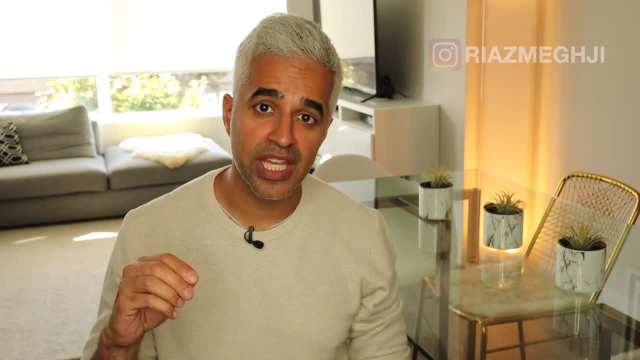 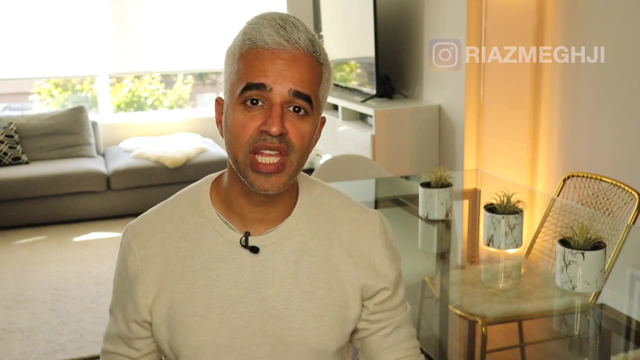 Determine who's in front of you and what you believe they need in this moment before you decide what you're going to say. You could even begin by literally checking in with the audience and asking them what they need or what they're feeling right now. 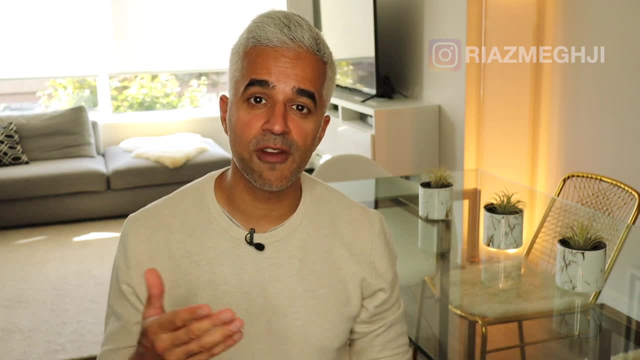 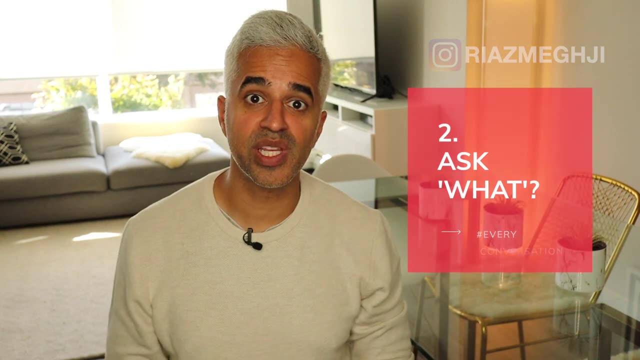 In some cases, this initial Q&A can make your presentation feel like a conversation and take the edge off What. Once you understand and recognize who you are speaking, to ask yourself what's the point you want to make or stance you want to take. 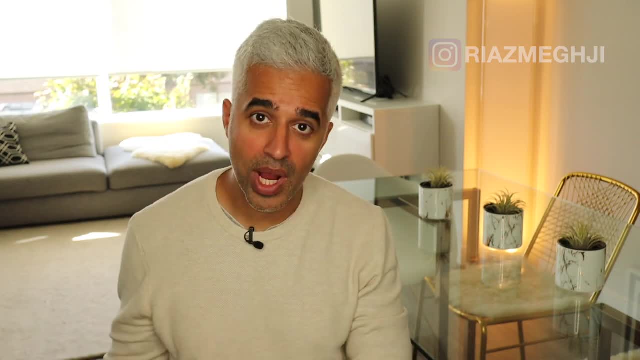 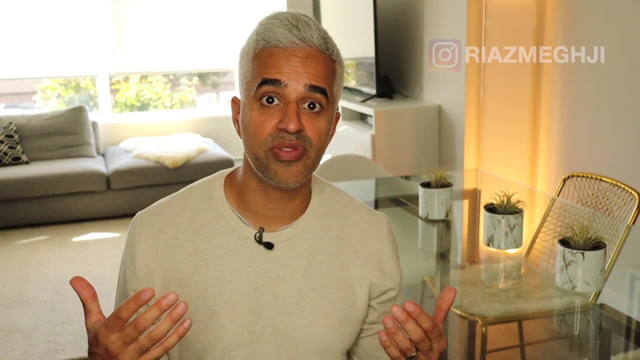 Either way, you want to make a powerful statement or ask a powerful question to grab their attention. For example, if people are struggling around you, you could make a point about why you believe things are going to turn around and become that beacon of hope for them. 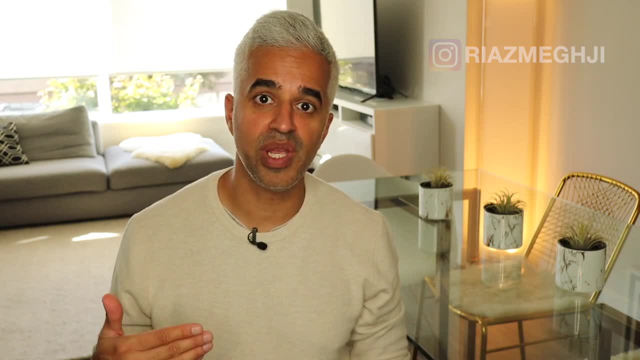 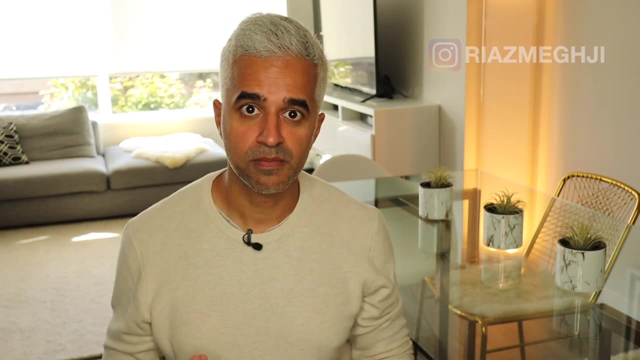 Be sure to give your audience an example or two to back up your ideas and opinions, to help make them believers as well. Another key question to ask yourself: what do I know? You could share your truth and start with a personal story that speaks to the audience's. 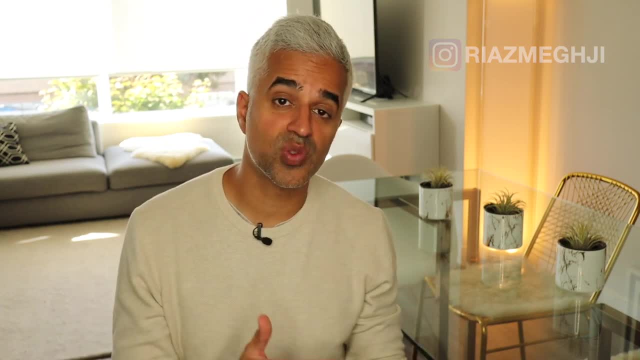 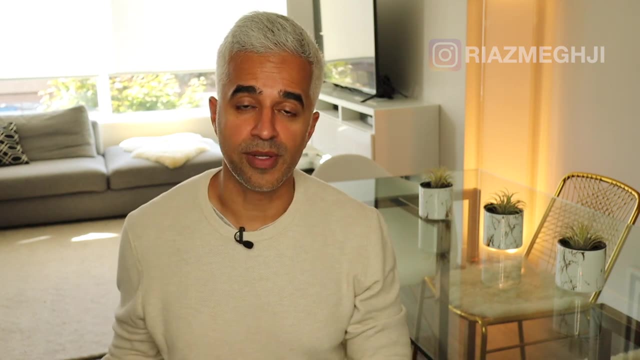 priorities. Storytelling can help put you at ease because, with events you personally experienced, it is so much easier to articulate the struggle, the conflict and the resolution. For example, with a year we've all had, in 2020,, for many there's a feeling of discomfort. 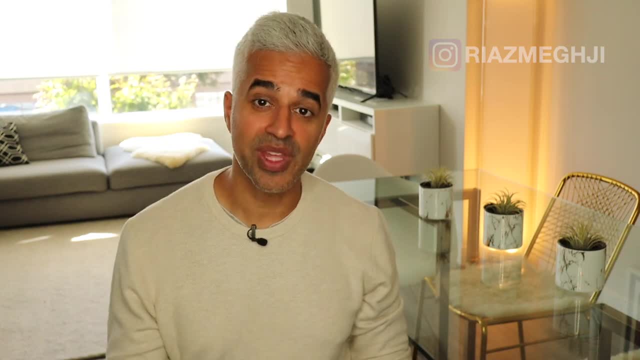 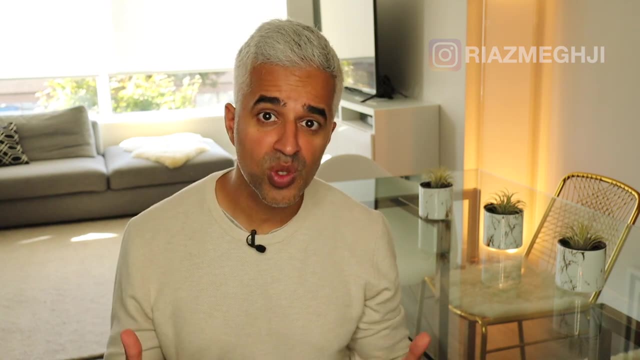 with the uncertainty about the future. Now, if you're making a claim that this disruption was what we need, What do you know needed to change habits and do things differently? you could share a raw personal story about how the new normal broke you down. then share how you worked through that adversity to create. 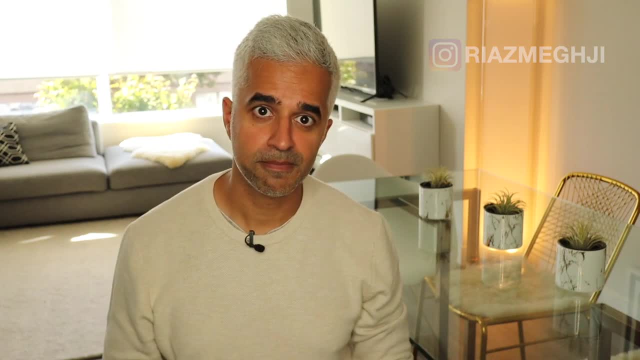 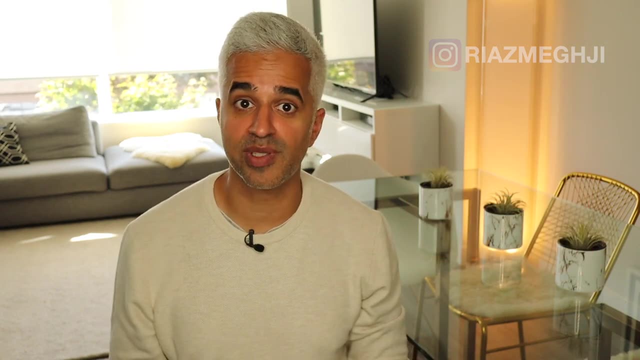 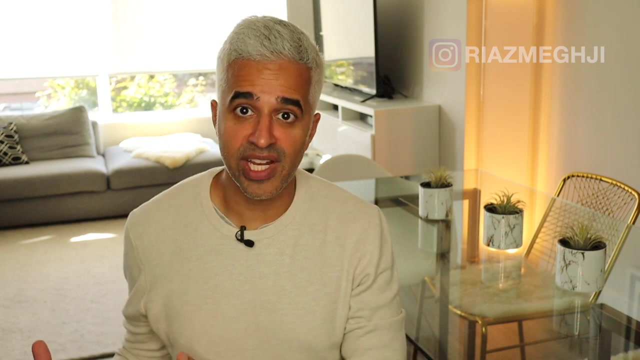 new opportunities for you and for others. Ask when. This is a great question to answer. to provide context. Your audience will always be curious about timelines When things happened. There could be a strong origin story to include here. When things changed, This could speak to the transition or adversity being faced or overcome. 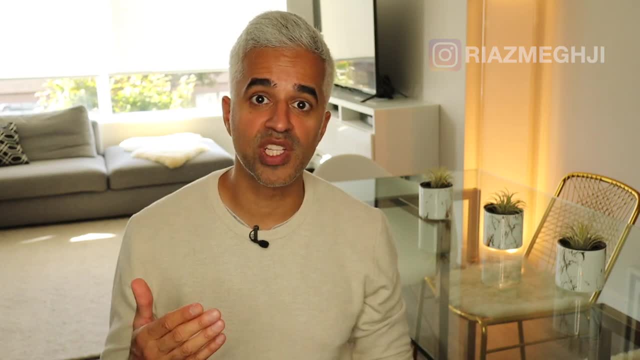 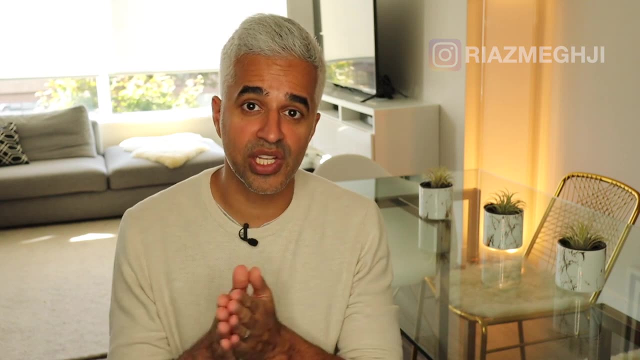 When things will be different? This is an important question to address for many people that may be struggling with a current reality. If you can help pinpoint a time when there will be a new reality or transformation, it gives people a perspective and schedule to follow. 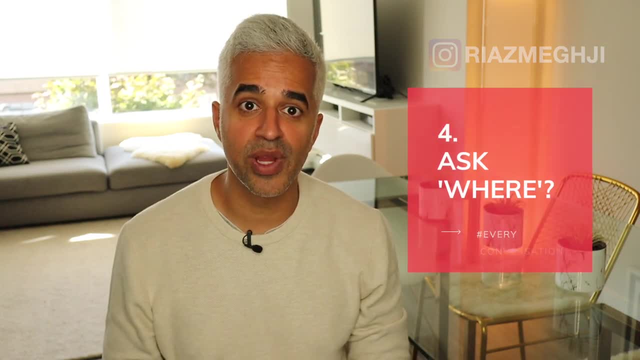 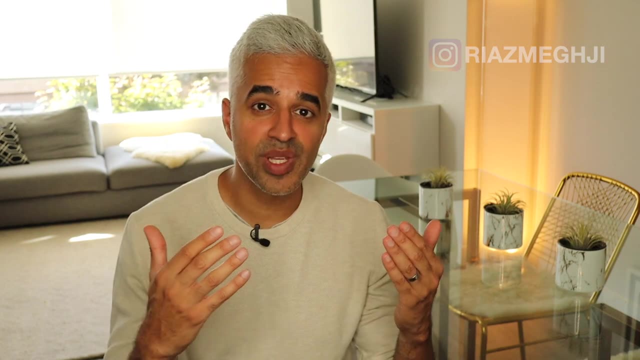 Ask where. Answering where allows you to speak to certain areas where things will be felt or be different. Where will things change? Where will things get better? Where things need to be explored. This helps you speak to specifics rather than making vague generalizations about what could. 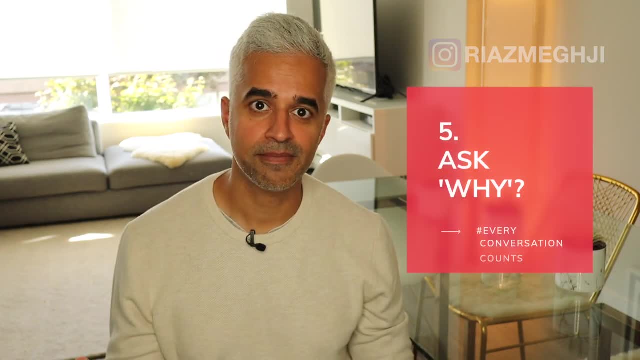 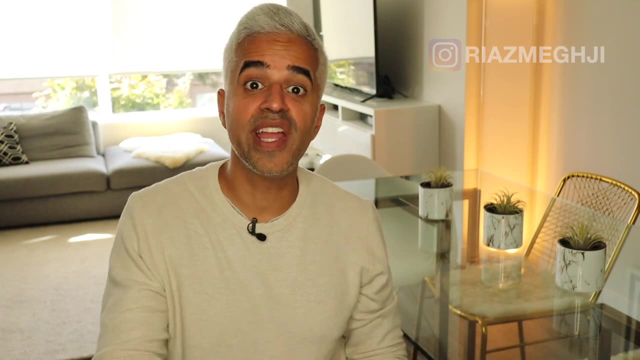 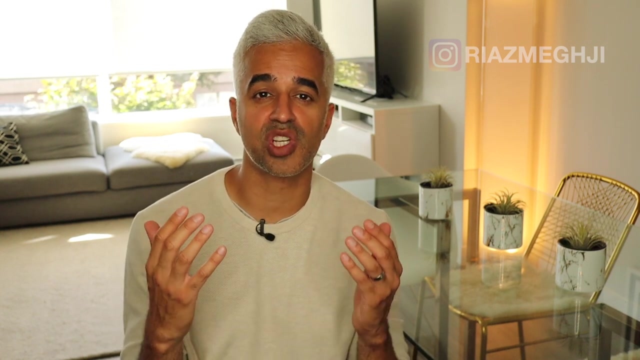 happen in the future And then ask why. This is a great question to answer as you complete your impromptu speech conveying your why, Why you care, Why they should care, Why they need to act now. These are all powerful questions to motivate your audience to do something with your message. 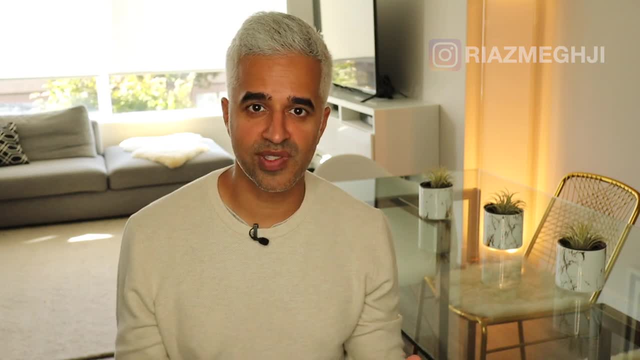 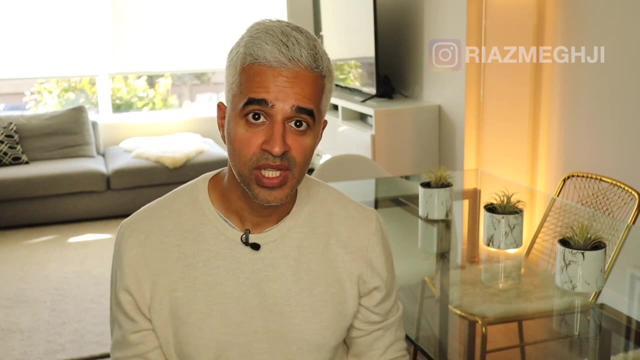 so they aren't just passively listening to you, but they're doing something with the ideas you're giving them. And closing out with the first steps for how they can take action is also valuable, And I'm going to throw in a bonus tip here. 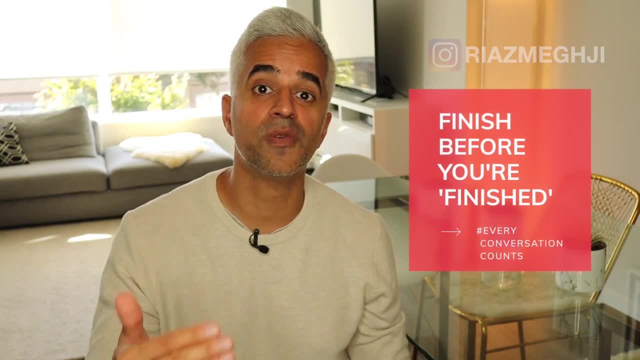 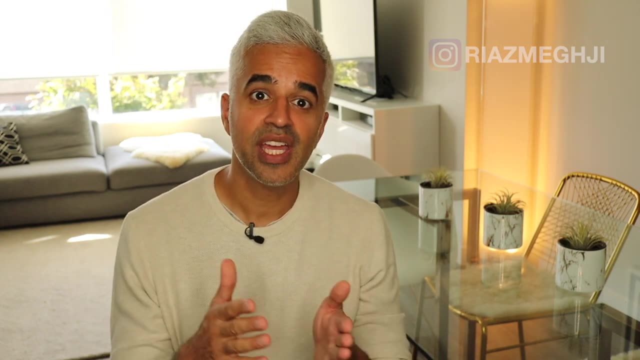 One of the most important considerations is to finish before you're finished. Don't speak until the point your audience starts tuning you out because you've gone on too long. Say what's needed and nothing more. If you think you won't have to deal with impromptu situations, consider this: 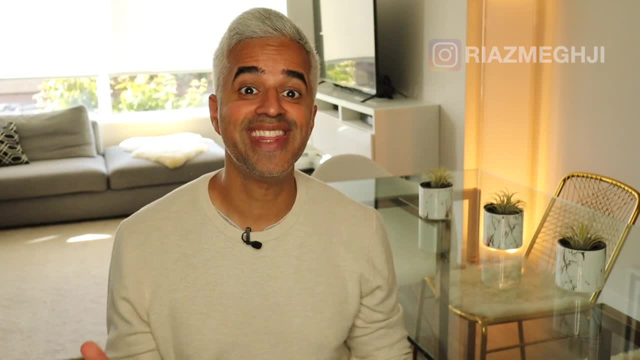 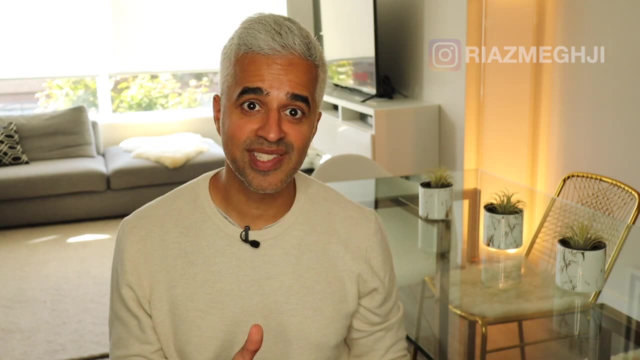 The better you get at delivering presentations that you've prepared beforehand, the higher the likelihood you will earn the job. That's it. You're going to get the trust of others and then be asked to speak impromptu, And mastering this skill gives you a competitive advantage: to be a trusted and articulate voice. 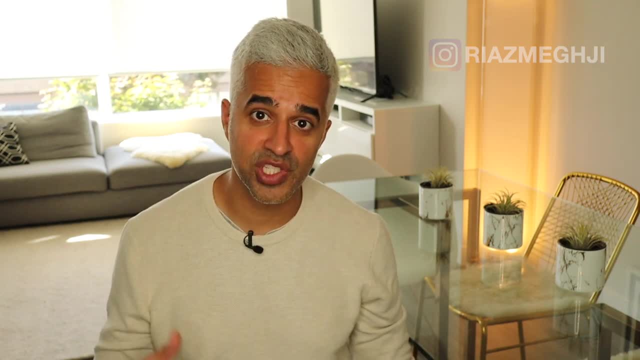 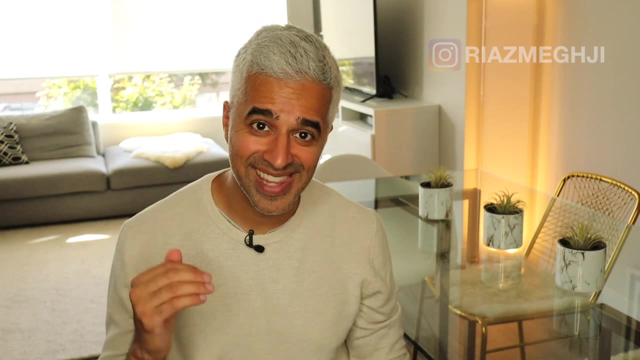 that offers value. If you use and answer these five questions as your framework, you will be able to craft something unique, something personal, something impactful and, above all, motivate your audience to listen to your every word. And remember, speaking is a game of follow the leader. 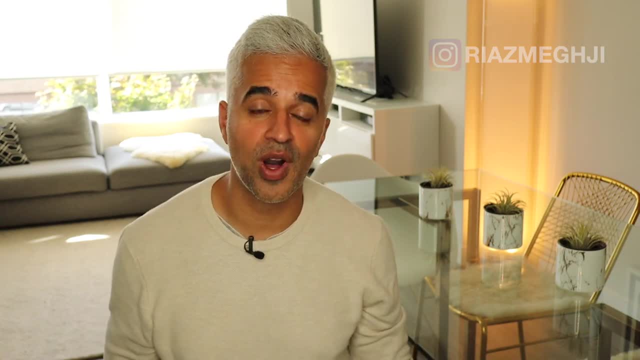 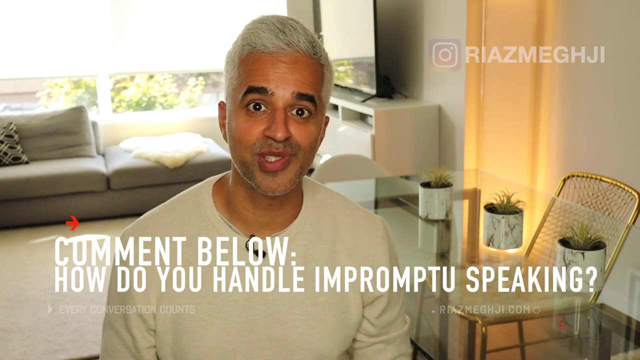 If you smile, if you laugh, if you have fun, The audience will follow you. Follow your example Now. how have you handled impromptu speaking in the past? Share your favorite tips and tricks for speaking without prep time in the comments below.